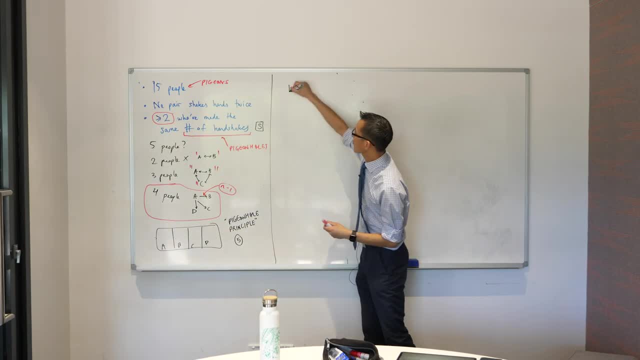 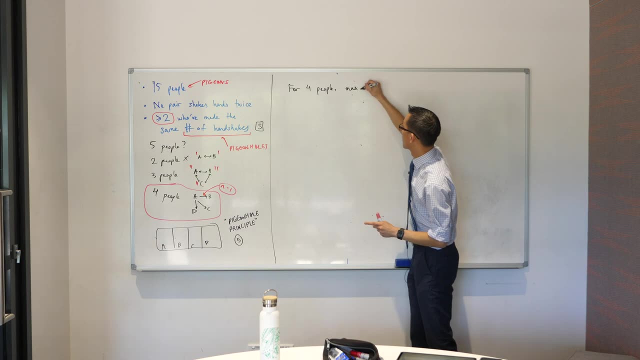 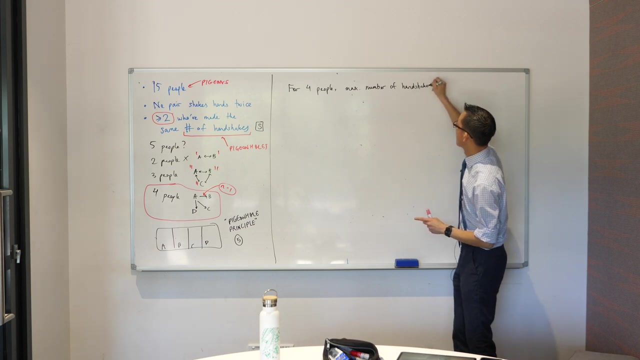 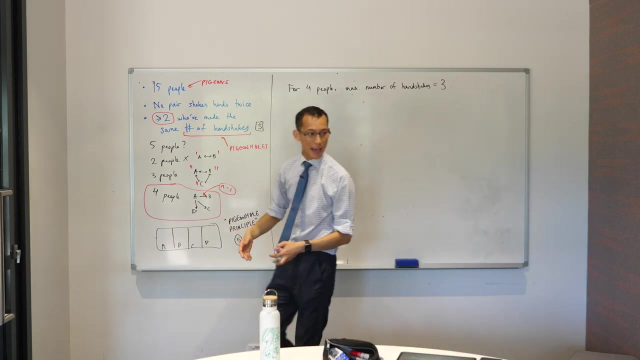 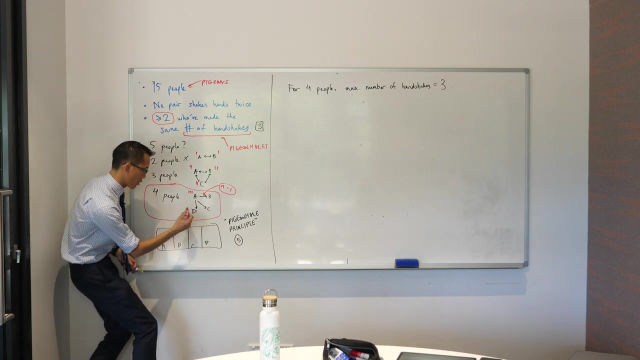 Okay. so therefore, I know, for four people, the maximum number of handshakes is what again? We just said three. So far, so good. If we actually went and played this out right. For example, in this situation, A is done. Let's tally it right: One, two, three handshakes. okay So far. 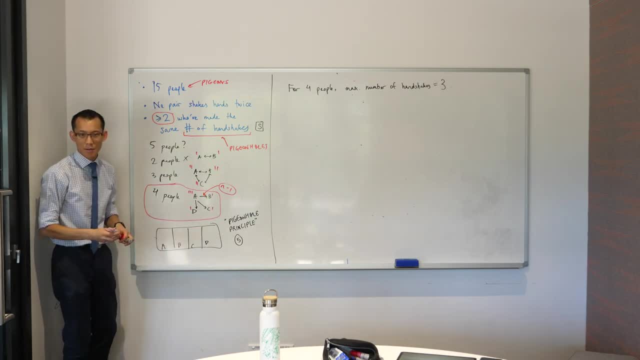 everyone else has just done the one. Is that okay? But think more stuff could happen right, Like what else could happen? Maybe C and D Shake hands. Where are we at at the moment? If I do that, they each have two now. okay, So more things happen right. And I suppose, if I wanted, 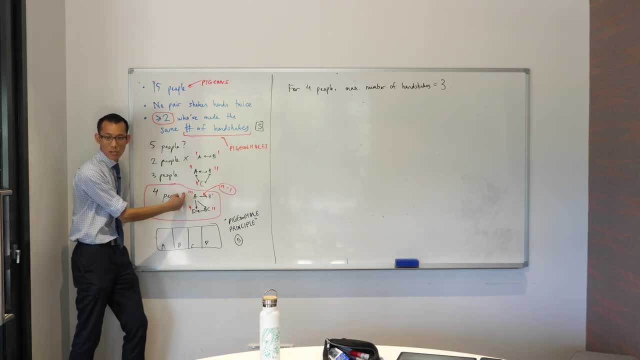 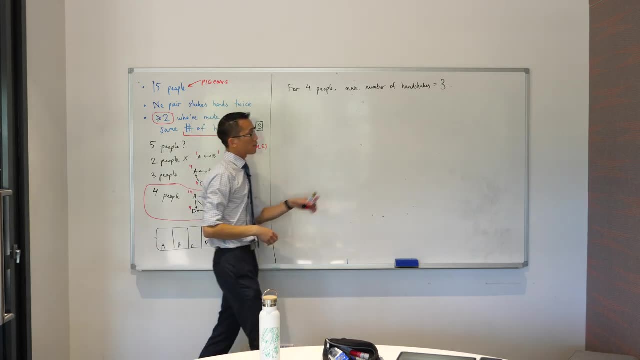 like, actually, at this point, all I'm going to do is get more people towards three handshakes. Does that make sense? Because these guys are already on two A can't shake hands with anyone else, right? So you could have three handshakes. You could have two handshakes You could have. 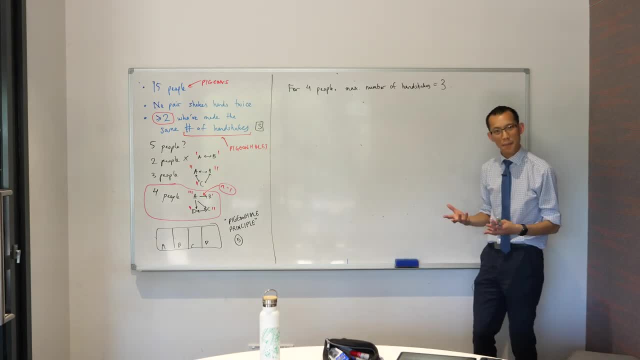 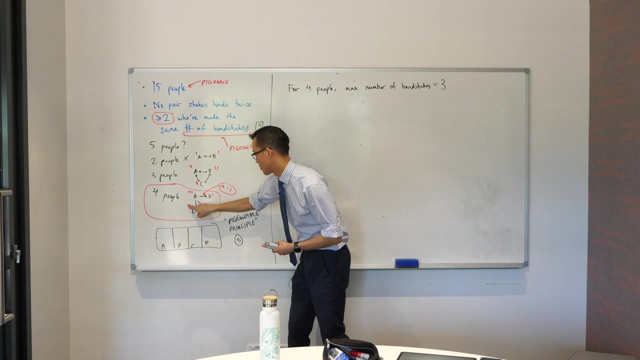 one handshake. So, in this situation, how many pigeonholes are there? Just having a look at this right, We know three is possible. If three happens, how many handshakes do all the rest of them have? Let me just rewind, go back to here At this point. if three handshakes, 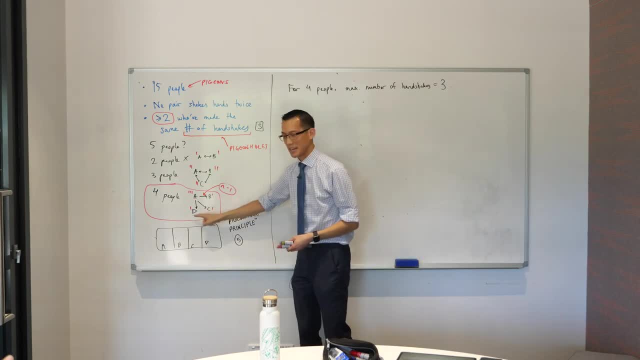 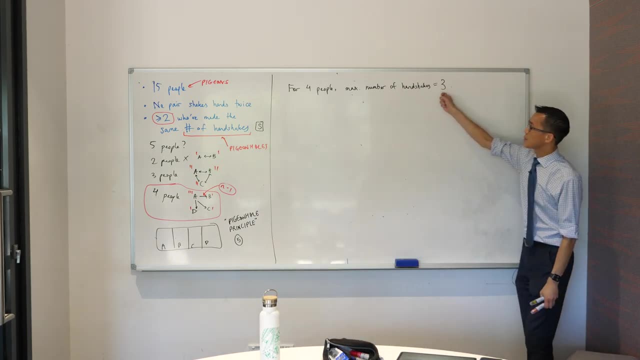 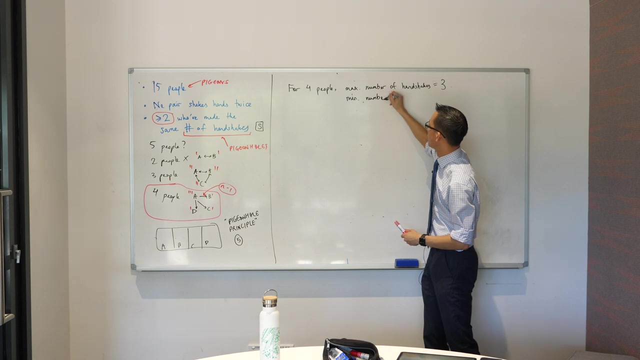 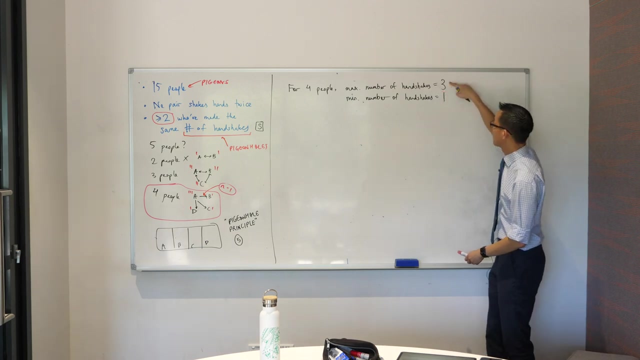 happen for A everyone's already at one Like that's: there can't be a person who didn't shake anyone's hand. Does that make sense? So therefore, the maximum number of handshakes here is three. The minimum number of handshakes in this situation is what It's one, Because we just said there was. 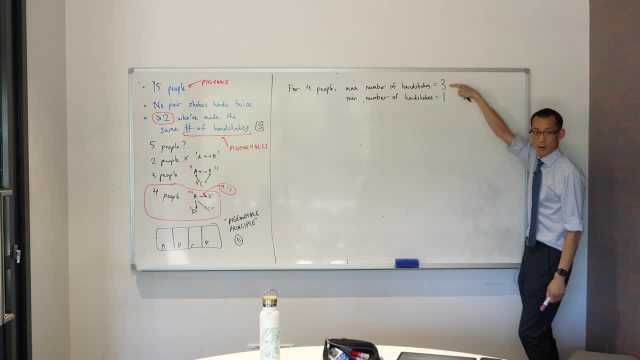 one person who shook everyone's hand because they're, I don't know, a social overachiever or something right. So in this case, have a look, right. And there's no such thing as a half handshake is there In this case? I know my pigeons. How many pigeonholes are there? 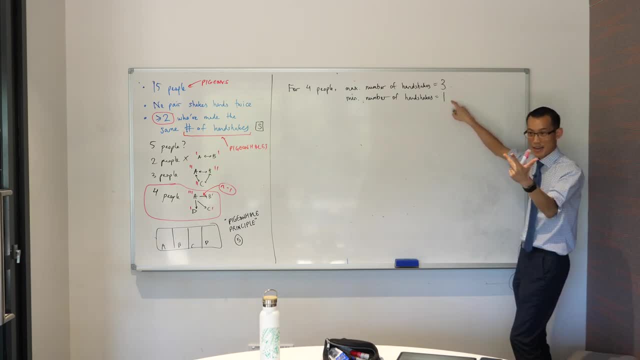 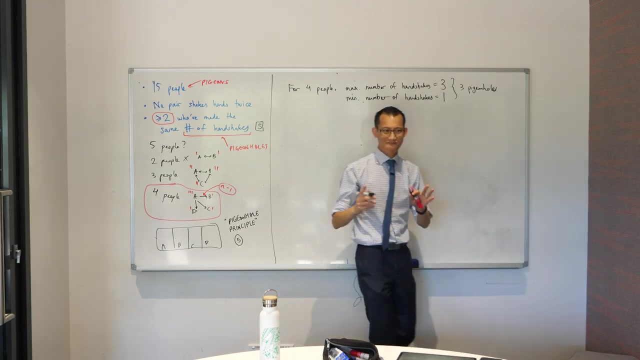 One or two or three. There are three pigeonholes. Do you see, what I've just established- Four pigeons, three pigeonholes- by pigeonhole principle, has to happen. okay, Now, this is a question. I'm going to ask you a question. I'm going to ask you a question. I'm going to ask you a question. 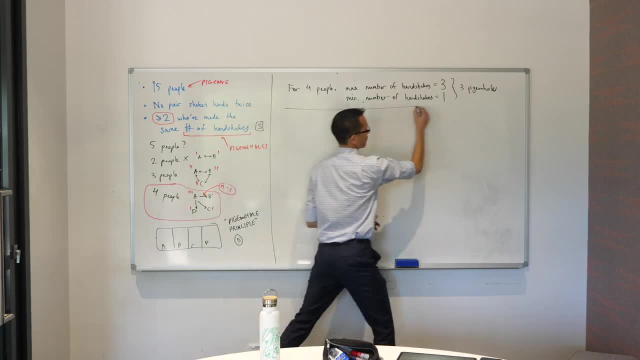 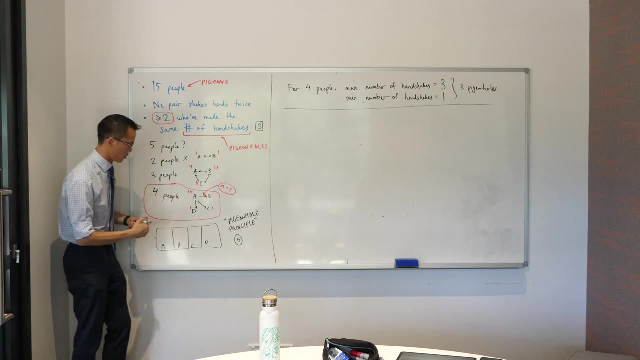 Actually, there's one other way for this to happen, though, because, remember, we said- like we just kind of played out- what's the maximum number of handshakes. that happens, but that's because A, for some reason, is just ultra extroverted and they made sure they got around. 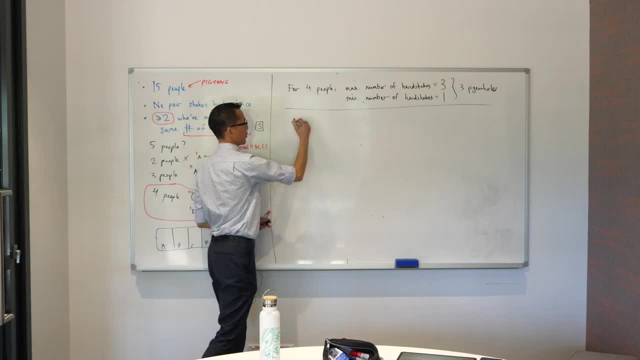 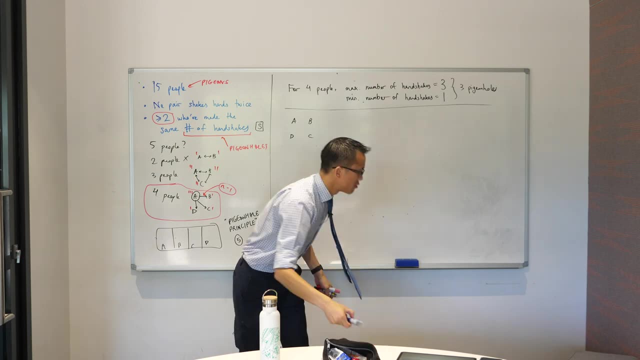 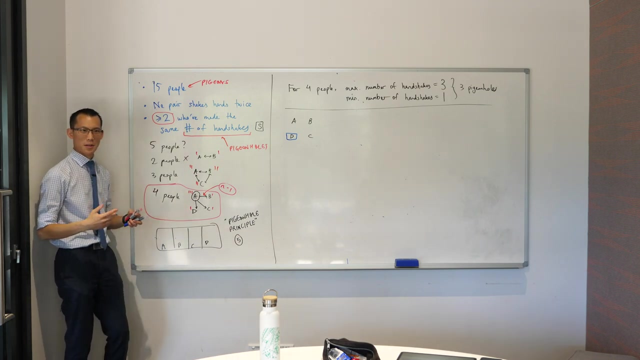 to everyone. okay, Let's just like replay the situation again. You've got A, B, C and D, okay, And maybe what you find is I don't know D, they're just super COVID, like aware or something like that, and they're like I refuse to shake hands with anyone, okay. 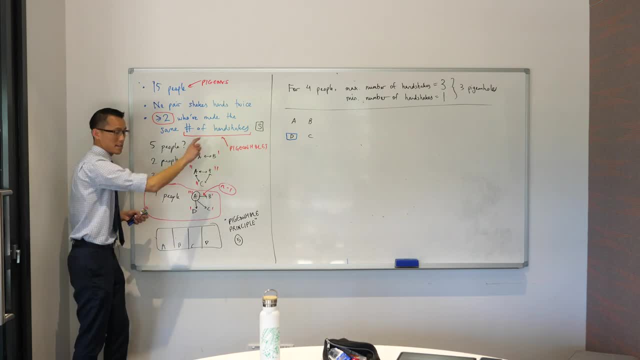 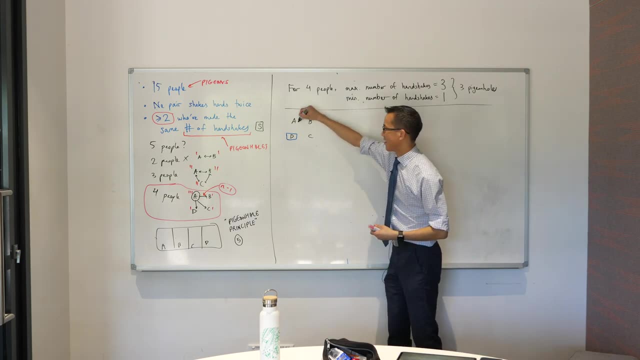 So now what happens? What's the maximum number of handshakes in this situation? It's two. Where'd you get two from? We went back with A being, like you know, very extroverted, right, So they shake hands with B. 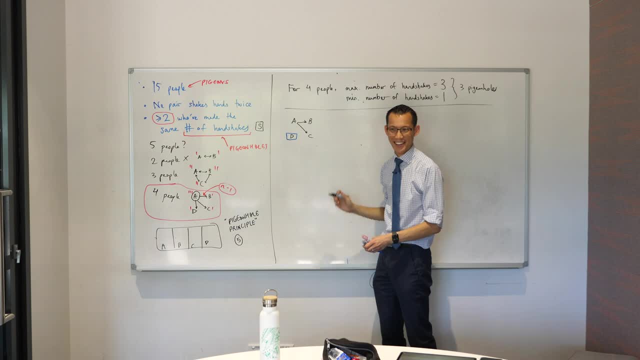 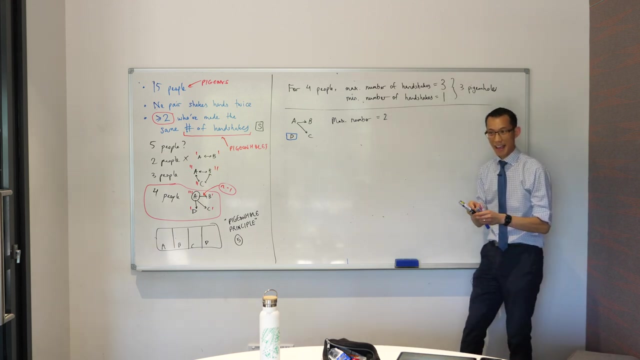 they shake hands with C and then they're like yeah, nah, right. So they just kind of like awkwardly elbow bump or something like that. So the maximum here is two. What's the minimum in this situation? It's zero because of this person who doesn't want to shake. 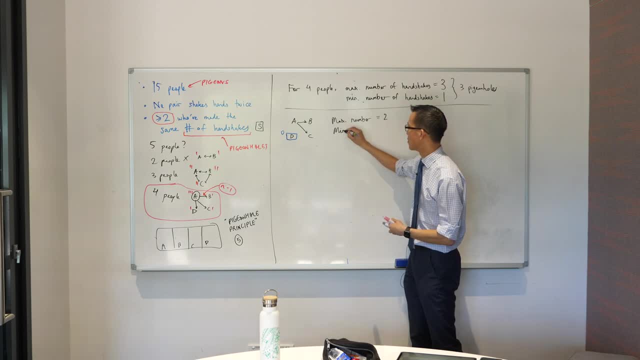 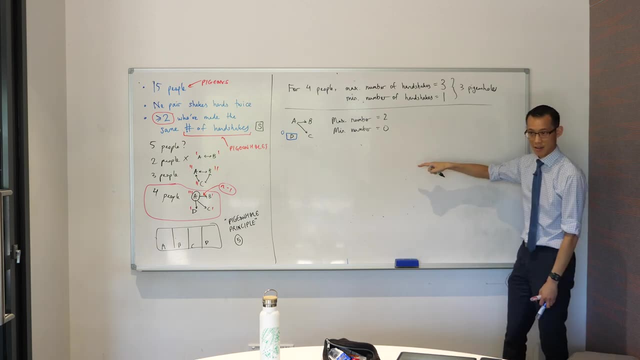 hands with anyone, right? So here the minimum number is zero. Okay, just like before, there's no half handshakes, right? So how many pigeonholes are there in this situation? It's either zero or one or two. 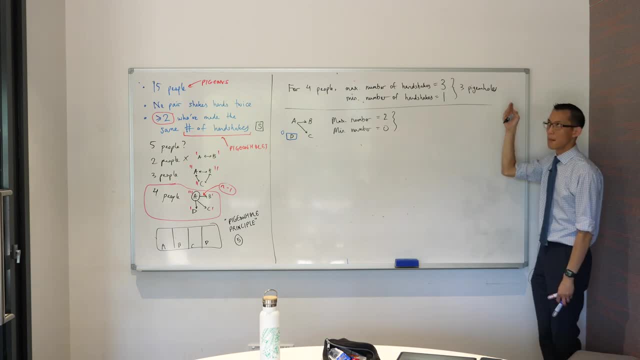 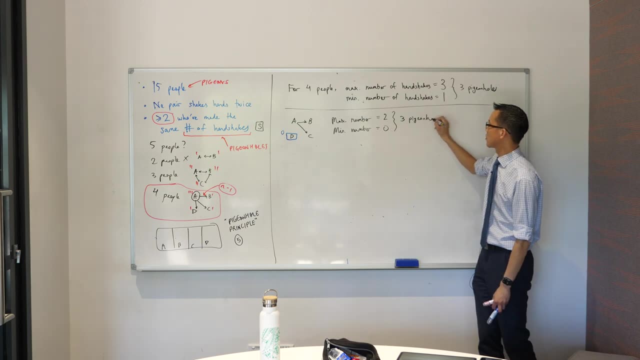 There's still the same three pigeonholes, or the same number of pigeonholes, even though the actual pigeonholes are different. okay, So this is still three pigeonholes for four people. Does that make sense? And that's why you can actually see the numbers right now. 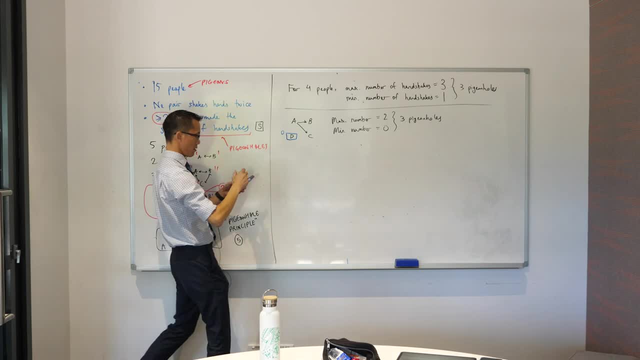 Have a look, right, I've got zero, and then, going back here, I've got two. one and one right, Like there's no way that B and C can't be. You can keep on doing it, right, We could go to five people. 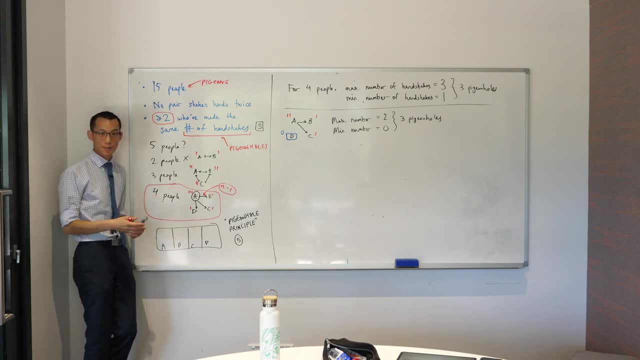 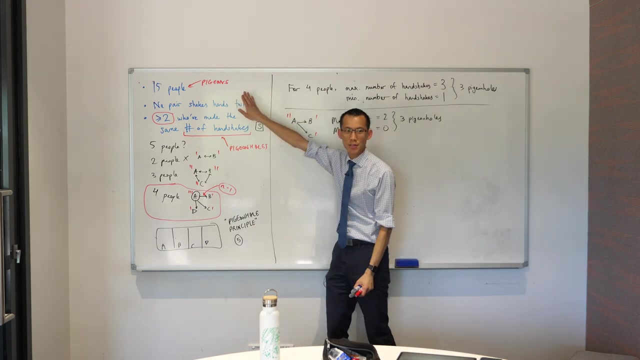 as you suggested, and you still will not be able to get two people having a different number. How's your brain feeling at the moment? Were you able to follow the argument? Let me just rewind right. The real key for every pigeonhole principle question is work out what are the pigeons and what are the 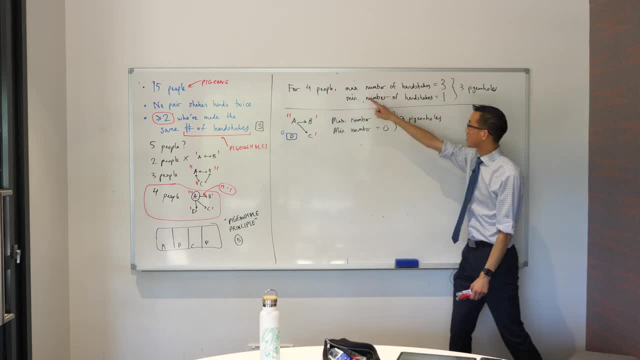 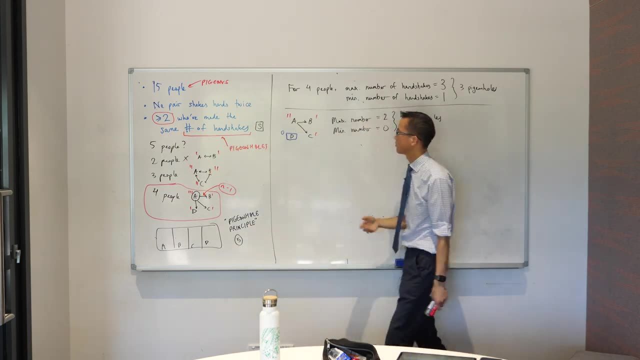 pigeonholes, right, And then, once you know one is going to be larger than the other, that's why you get this pairing happening, or at least pairing okay. So I'm just returning back to that. That's the principle, And any question you can throw at me. 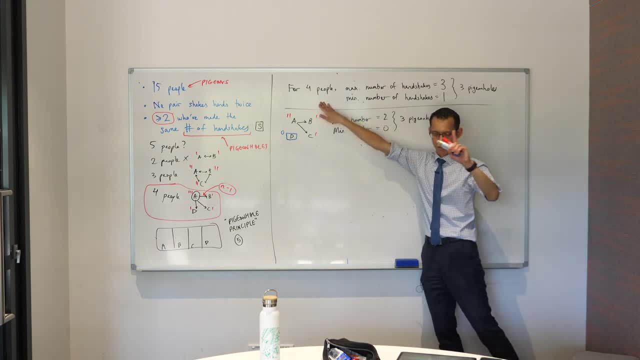 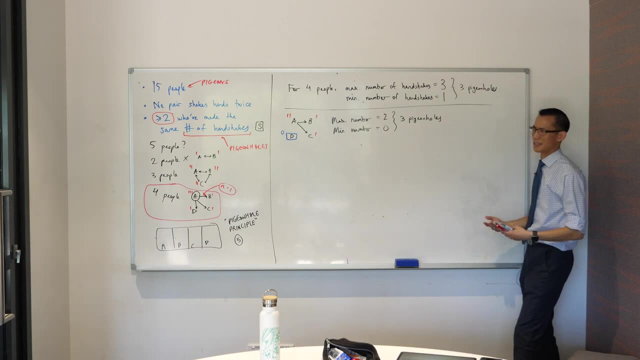 I just want to identify what has to match up to what other things, So people and number of handshakes or number of friends on Facebook, or- Sorry, that's a really old thing- Like whichever thing Shows my age, Whichever other thing, like number of donuts that they've eaten right, Or 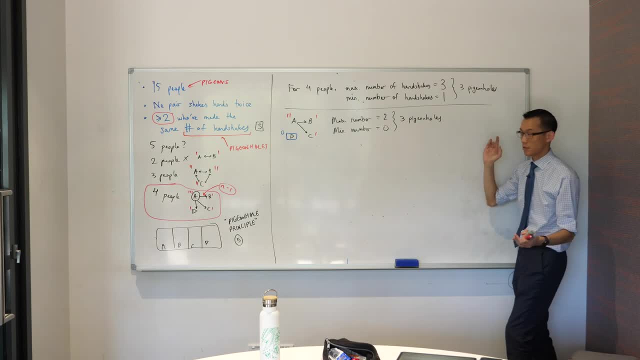 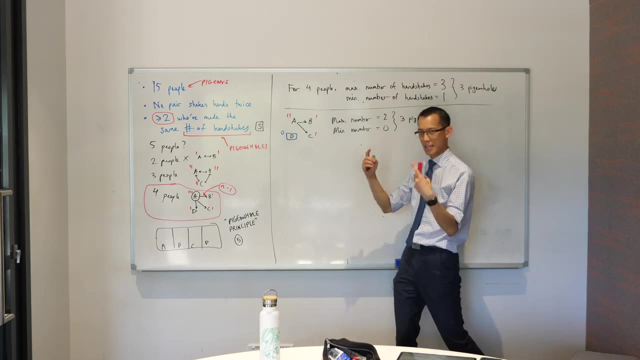 how many cities they visited in the world So long as like if I've got Like. this is the same reasoning underneath how I can know that there are at least two people who have the same number of hairs on their head in Sydney. 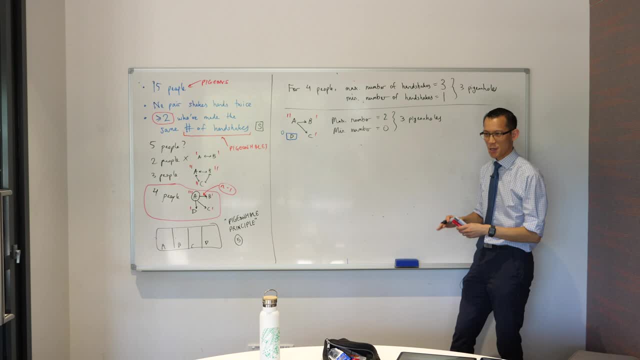 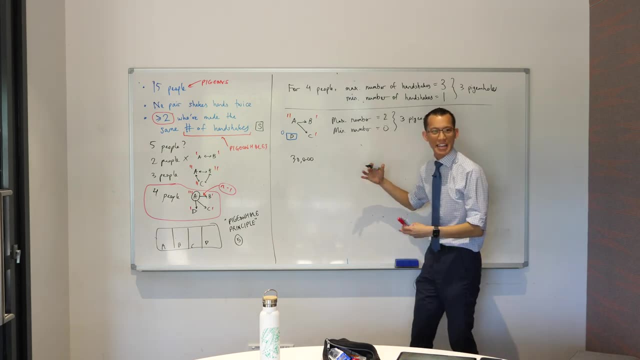 Have you heard this before? I've heard the other question. Yeah. So what they would say is, like the person who's got the most hair on their head. it's something like 30,000 hairs, which doesn't sound like actually that many. You're like: I feel like I've got lots right. 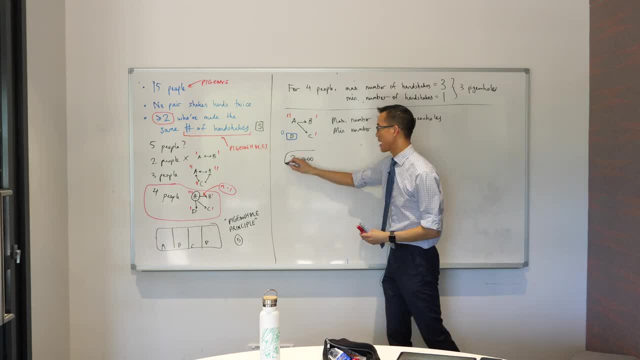 It's just the area of your head and how thick a human hair is right. So 30,000, right, And obviously there's some person who has no hairs on their head- right. But if you've got 30,000, then you're going to be like: 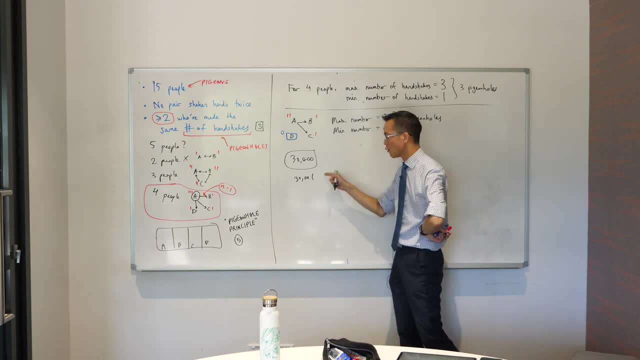 100,000 people. If I've got 30,000 and one people, at least two of them will have the same number, right? Maybe it's that two bald guys. That's fine. In fact, Sydney has like over four million people, right. 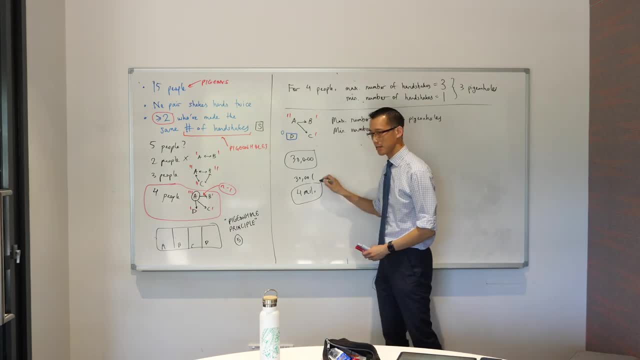 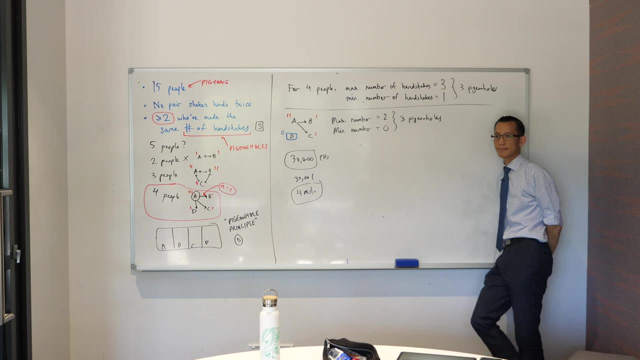 So you got loads and loads of people who have that same number of hair: pigeons, pigeonholes. That's all there is to it. Okay, Could you Like give example of a concluding statement Like communicable things, Sure, Yeah, Okay. 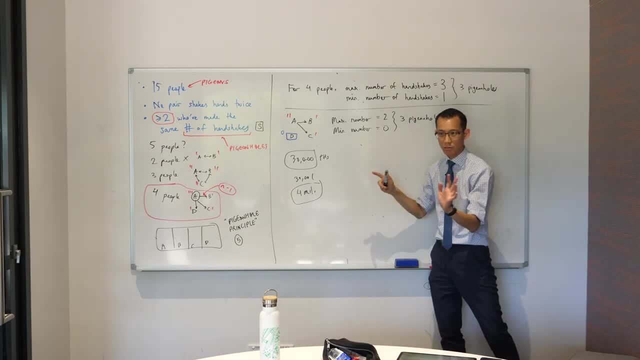 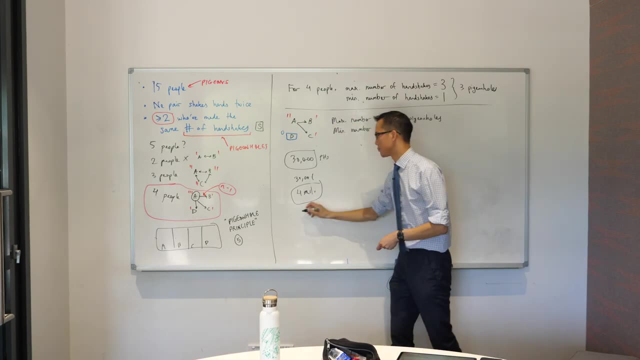 So I would say so what we've done is we've just modeled everything right, And what we've got here is we've established that for these smaller cases, right For n people, there are n minus 1 handshakes possible. 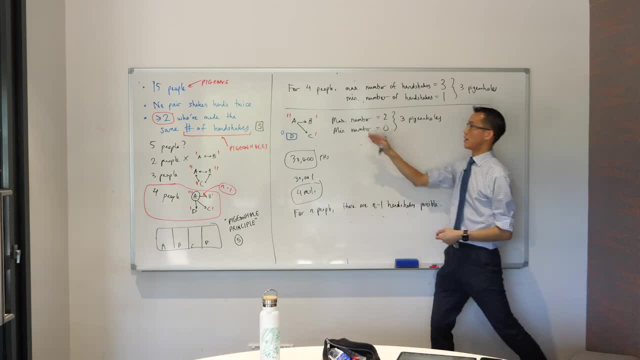 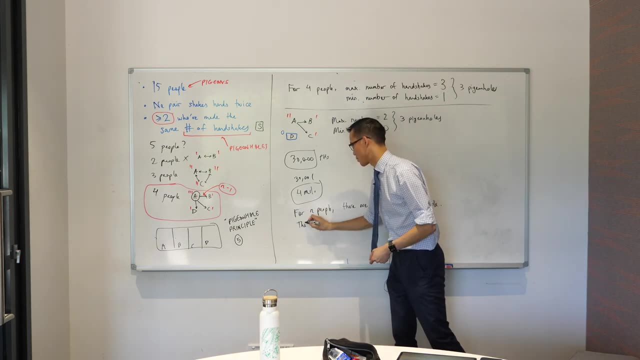 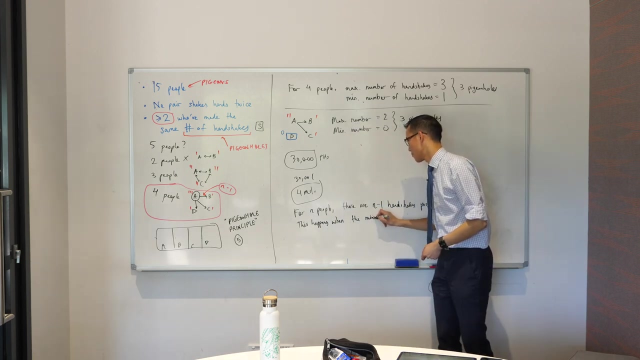 Okay, that's what I kind of got to up here. So you said: 4 people, 3 handshakes possible. Well, this happens when, or this occurs when, the minimum is 1 handshake, And this is where I've reasoned that right. 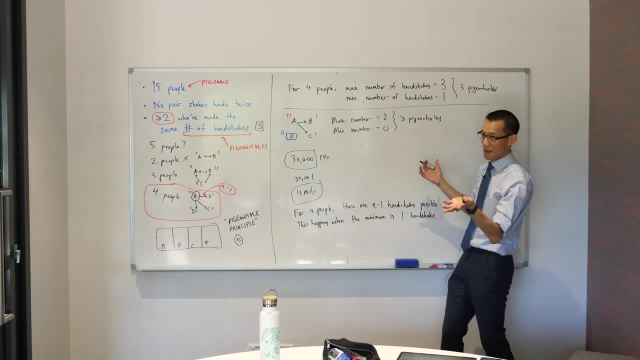 This is, and unfortunately, one of the things about this part of maths is it is a little bit wordy because there aren't. I mean, I could give you symbols to represent all this, but actually the symbols would be worse. At least words I understand, right. 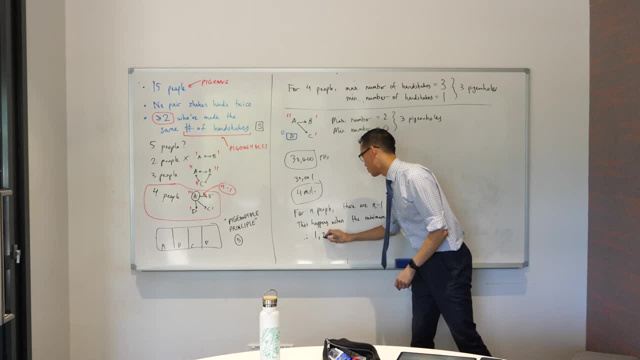 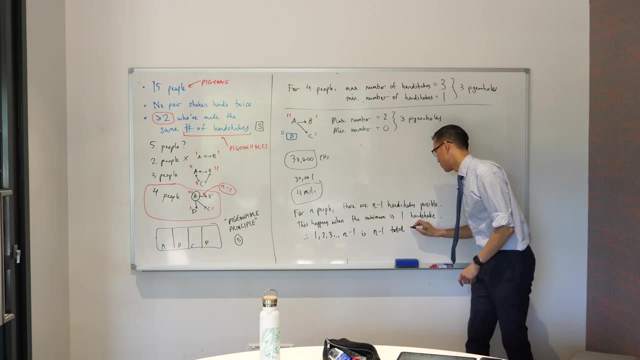 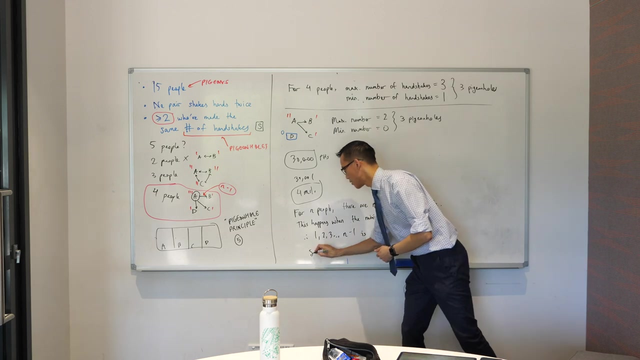 So I can say, therefore: 1,, 2,, 3,, dot, dot, dot to n minus 1 is n minus 1 total pigeonholes. So by the pigeonhole principle I would actually write the words pigeonhole principle, by the way. 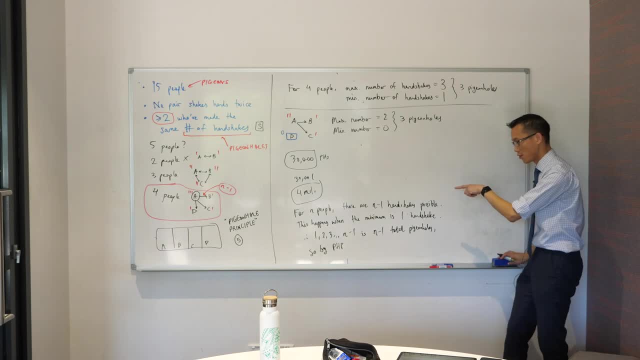 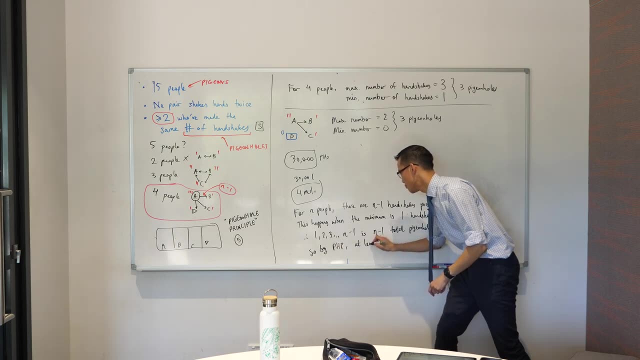 but I'm just I'm trying to save you guys a bit of time so you don't have to wait for me. right, By the pigeonhole principle. what have I got here? At least 2 of the n people, and in this case, like it could be 15, or it could be 4,. 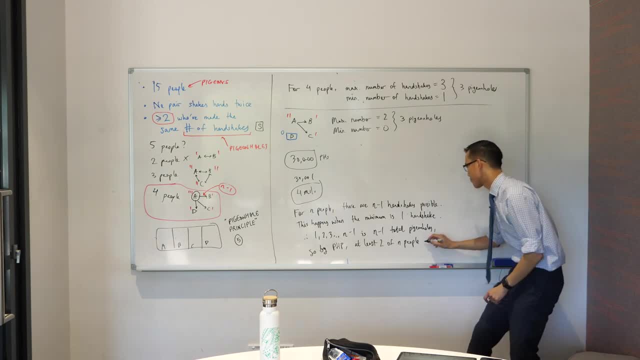 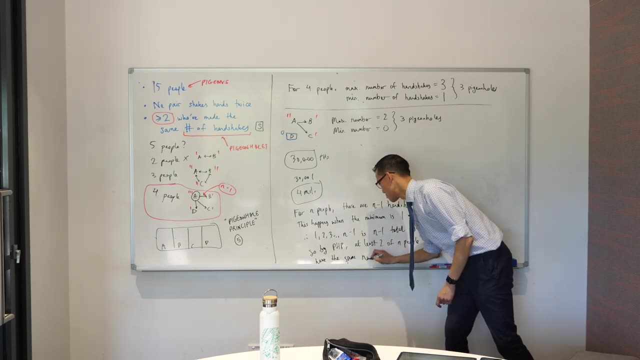 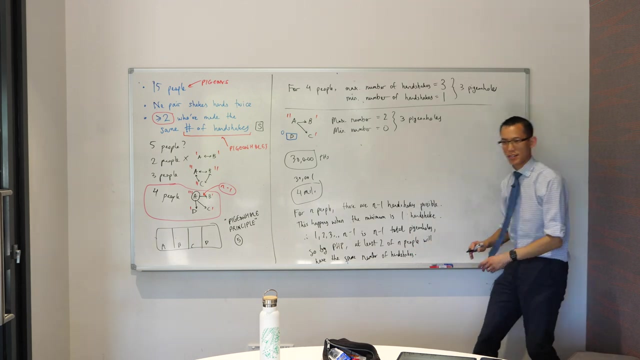 or it could be 700, right? It actually doesn't matter, We'll have the same number of handshakes. Sorry that handwriting is so horrendous, But there's the idea, right. So all you really need to establish is: well, you have to say pigeonhole principle somewhere. 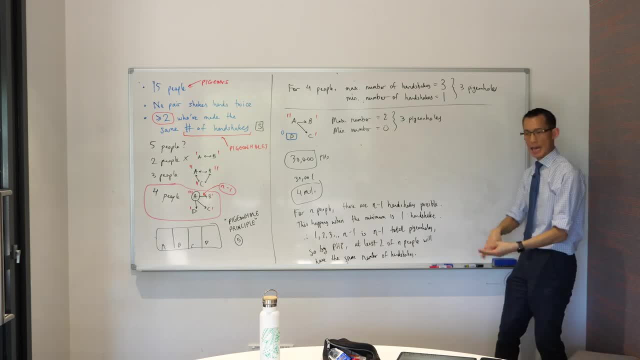 It's a bit like mathematical induction in that way, Like I've got to use the phrase. And then, secondly, the key idea is: where did I have it? Pigeons versus pigeonholes? That's it. That is the pigeonhole principle. 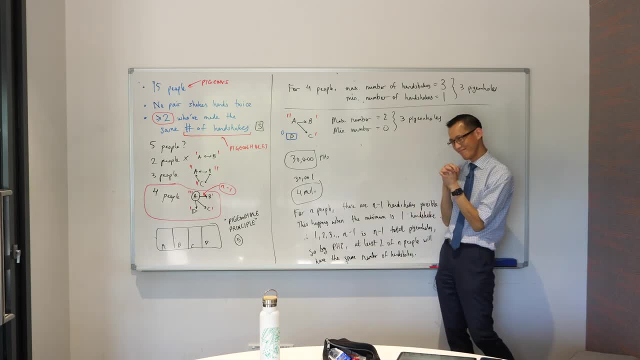 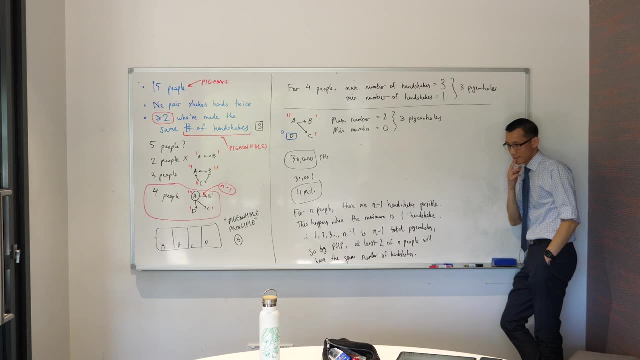 So long as one is more than the other, you'll get some pairing somewhere, Is that okay? I have two questions. Yeah, go for it. Why, when the minimum is 1?? Because you did in the example above, the minimum is 0, and you still got. 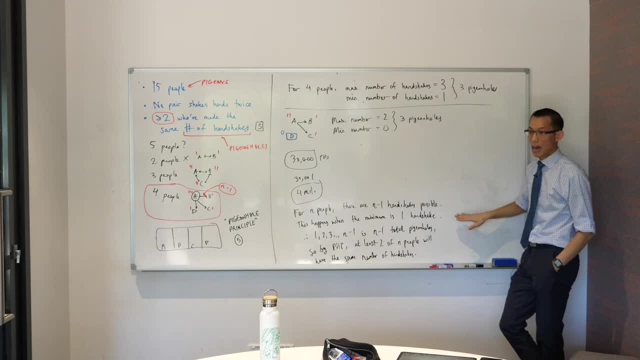 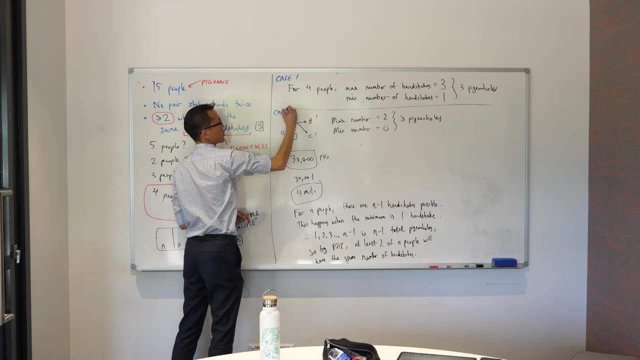 Yep, Okay. so then what I would say is, like I would have this. This is actually- I'm glad you mentioned it. actually, This is two separate cases, So I'd call this case 1, and I'd call this case 2 in my working right. 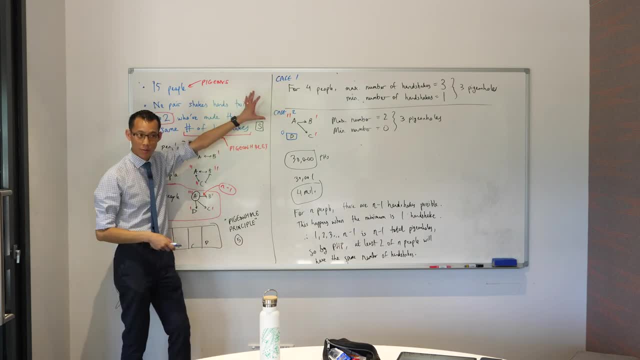 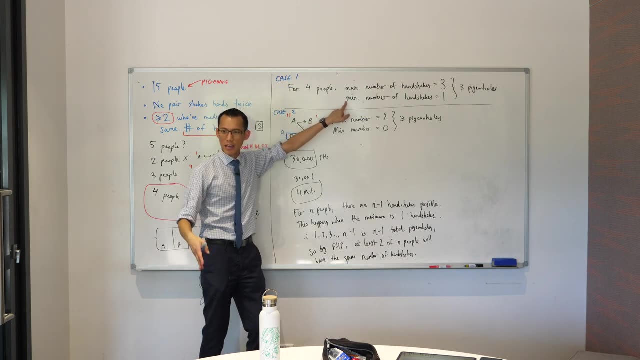 And so, no matter which one I go for, like these are the only two possible things. I guess what I'm trying to do is say: how high can that maximum go? That has its own minimum Minimum associated with it. And then I say: but can I get any lower than this minimum? 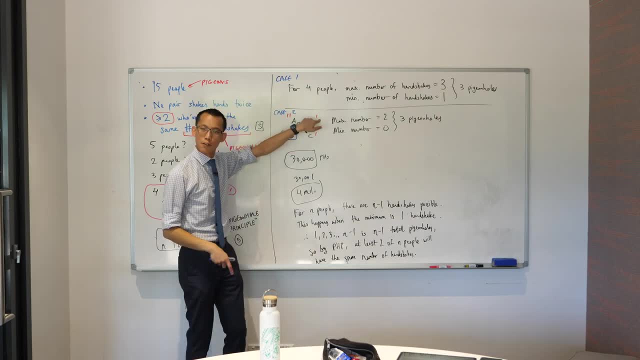 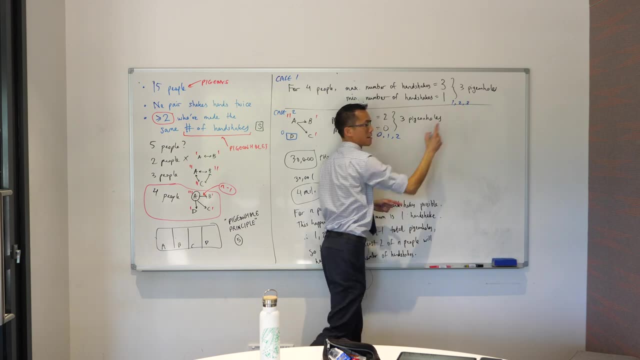 And the answer is: I can, but that minimum has a different maximum associated with it, So it's either 0, 1, and 2, or it's 1,, 2, and 3.. But in both cases, actually, it doesn't matter how many handshakes there are. 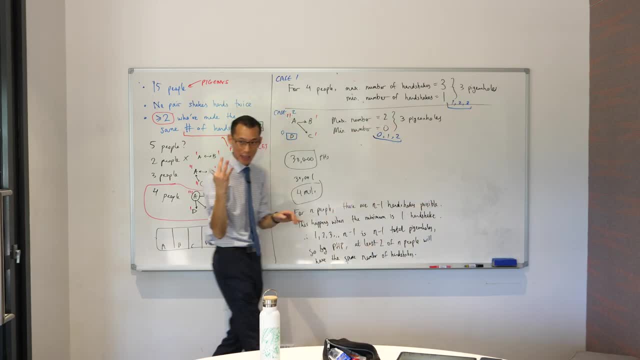 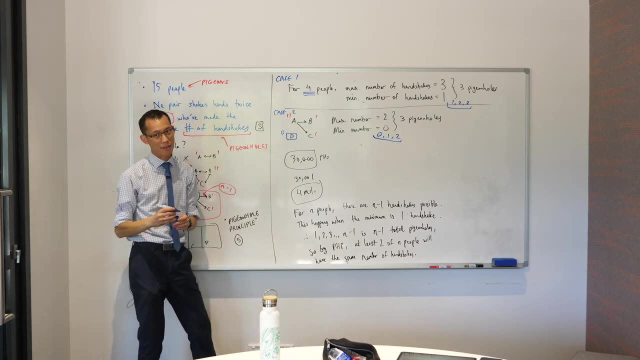 It matters how many pigeonholes there are. In both cases it's 3.. In both cases it's fewer than the number of people or pigeons that I have. As long as I've got fewer, it's okay. So I'd actually. I could write all of this again. 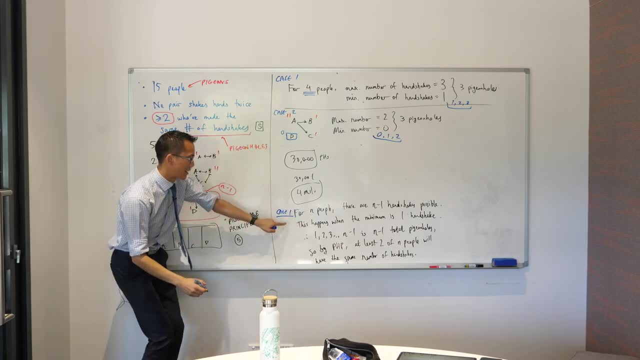 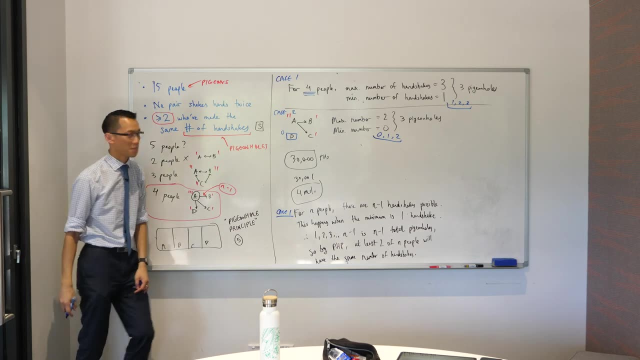 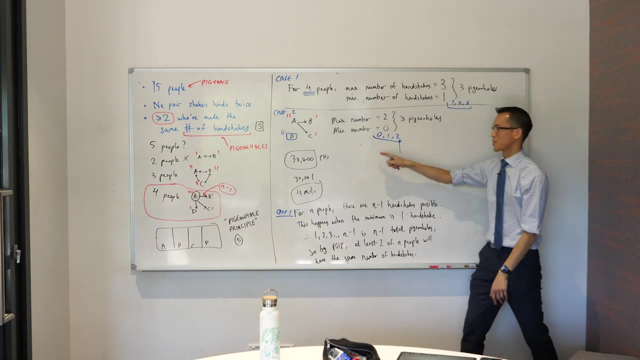 This is case 1.. I could write all of that again, but with n minus 2 and 0.. Does that make sense? Wait, why n minus 2? That number right there. So this is in that case where we've got some super antisocial person right. 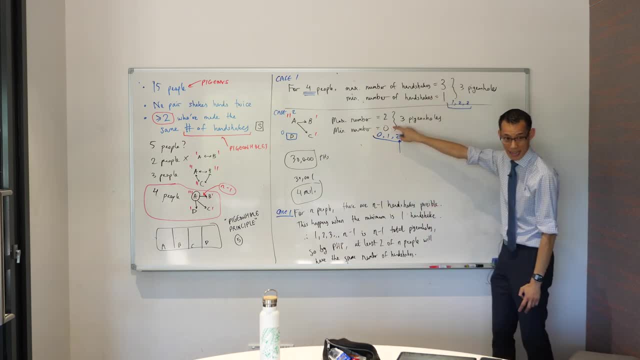 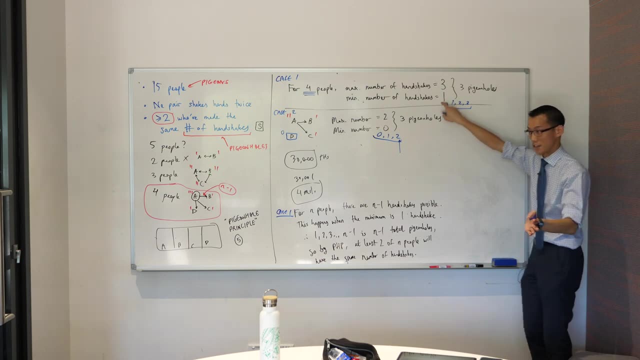 If you've got a super antisocial person who refuses to shake hands with anyone. so now I know I'm not in case 1.. That's how I know I'm not in case 1, because I've got someone who's got less than one handshake. 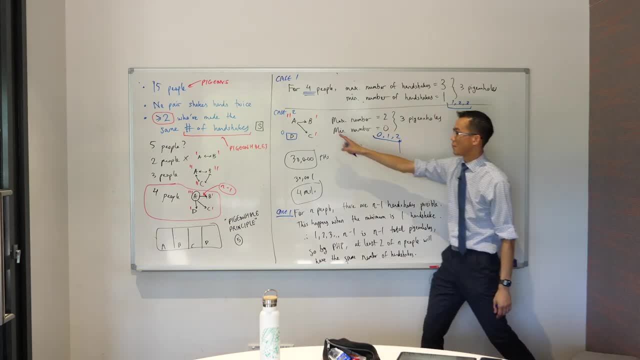 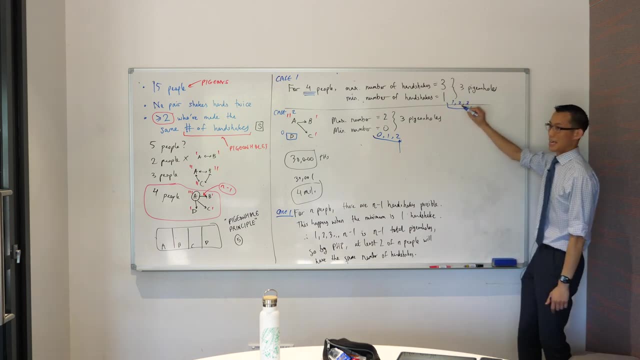 When you've got zero handshakes- though we had a look at this picture right here- The highest this can go is n minus 2.. So long as they can shake hands with everyone, that gives you n minus 1 handshakes. 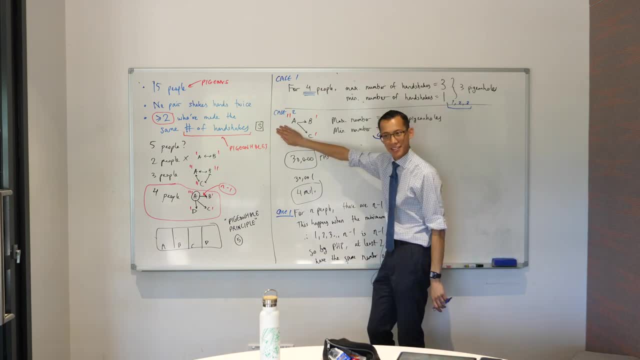 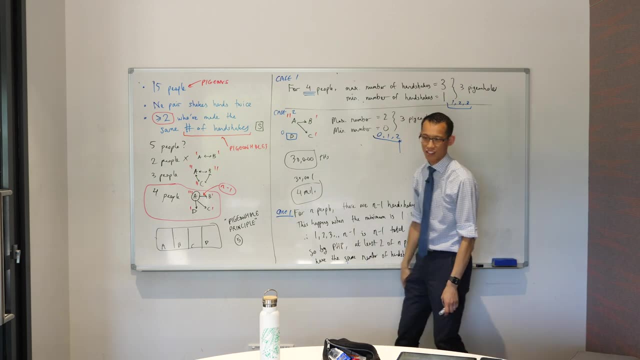 But if there's someone, it's actually like there's not that person in the situation. Does that make sense? So it's like: oh no, there's only this number of people there, 2.. But the total actually is 4.. 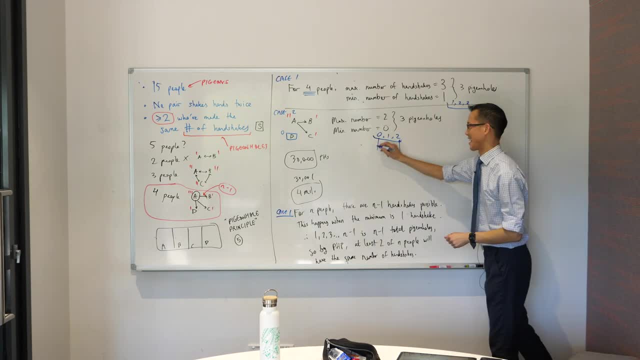 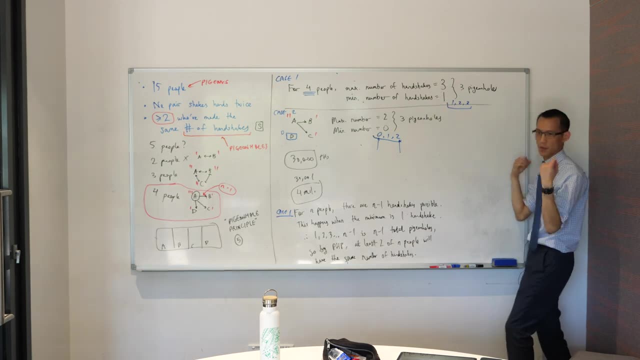 Okay, I know that's a bit tricky. It's the language around it and the fact that there are cases If it makes you feel any better. a lot of pigeonhole principle questions actually won't have different cases, They'll just be the one situation. 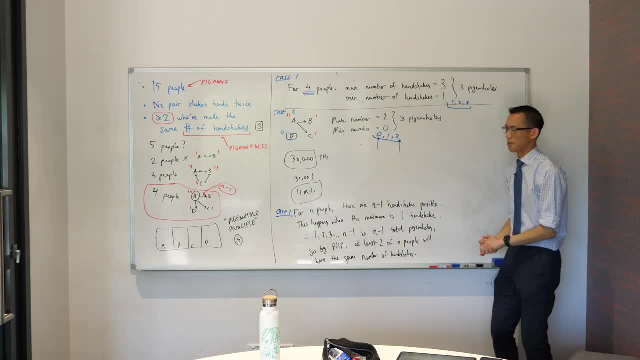 Work out how many of these, how many of these You're done? Okay, But this was a particularly maybe. this is why this was the example that was challenging for you to understand. Okay, So then for this, the actual question itself. 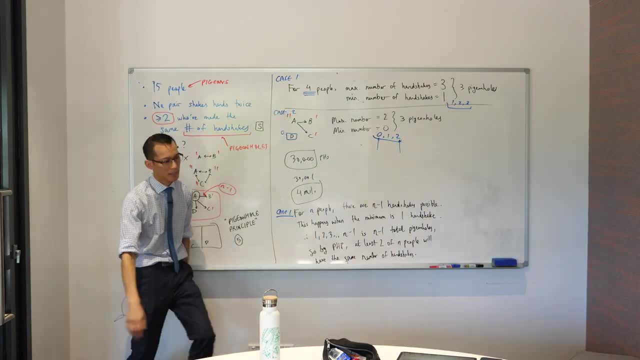 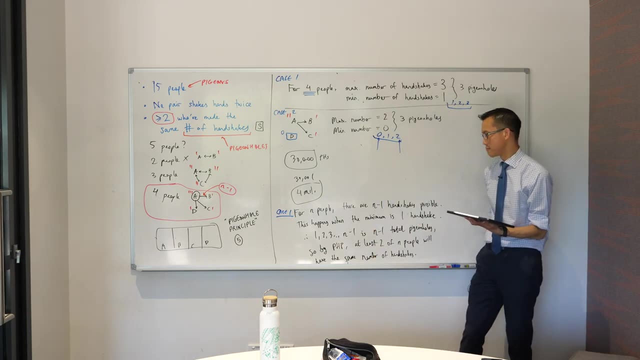 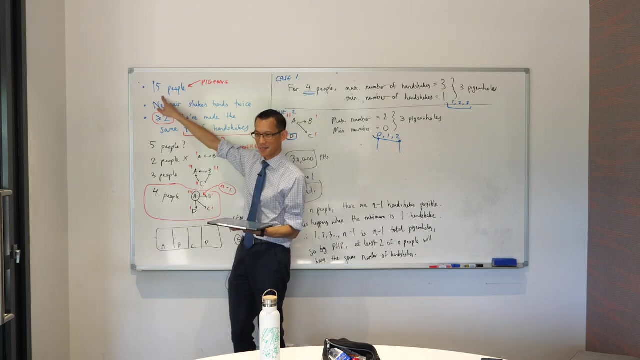 what was it asking? It said: prove that there will be at least two people who have made the same number of handshakes. Oh, so we don't even need to, Okay, Yeah, In fact it's kind of a total red herring is the technical phrase. 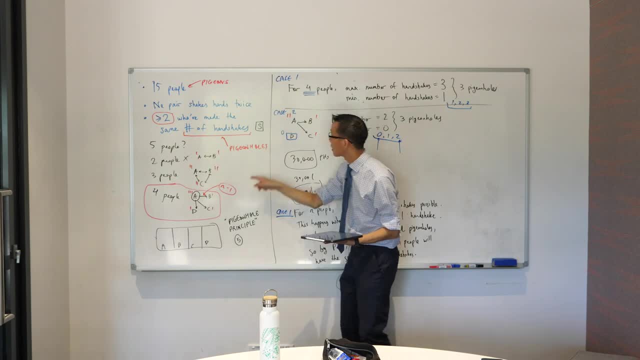 Like it's just a distraction. It doesn't have to be 15. as we've just demonstrated, It actually could be any number so long as it's well. in fact, not even so long as it's more than one person, they'll have the same number. 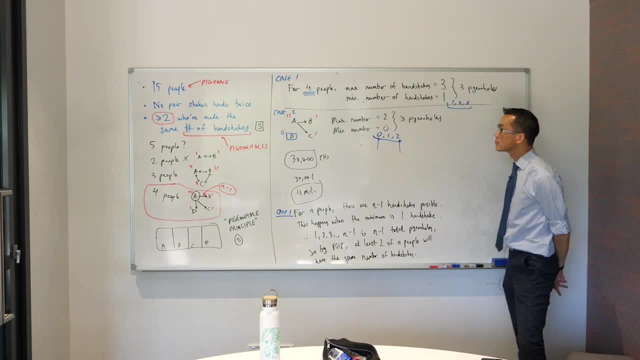 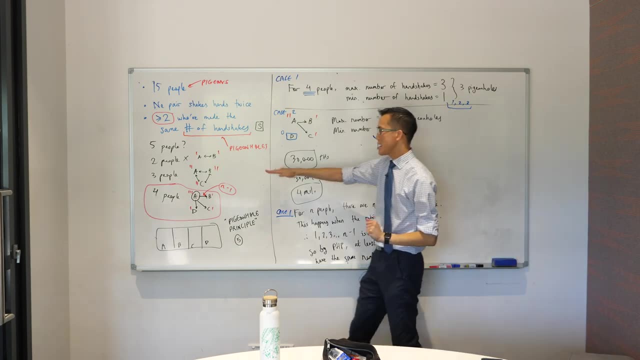 So if I was in an exam situation and I did like what you did here with 2 people, 3 people, 4 people, would that be okay? So it would be okay as a start. So me doing this was my way of understanding. actually, this is what I wanted to establish, right. 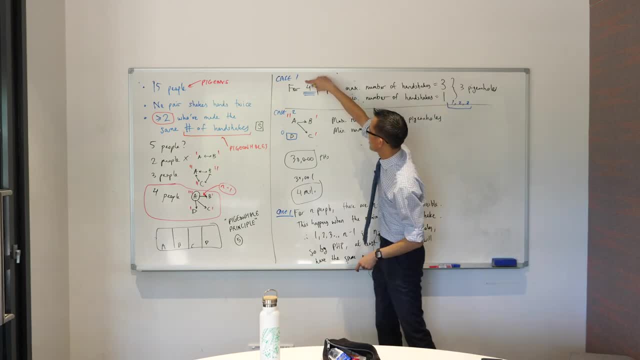 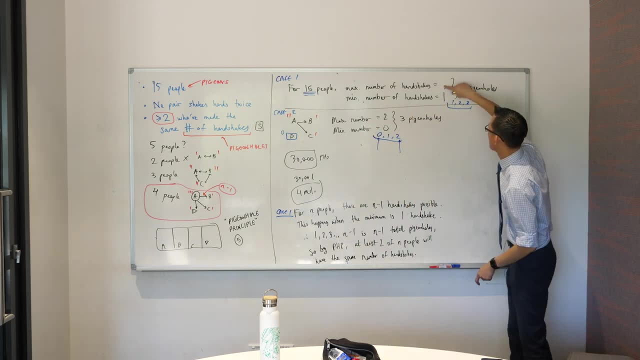 So probably a better way that I could have done this is actually to go all the way up to 15. at this point I've established a pattern and then I can say it's going to be 14 and then 1. And then here it would be again for 15 people. 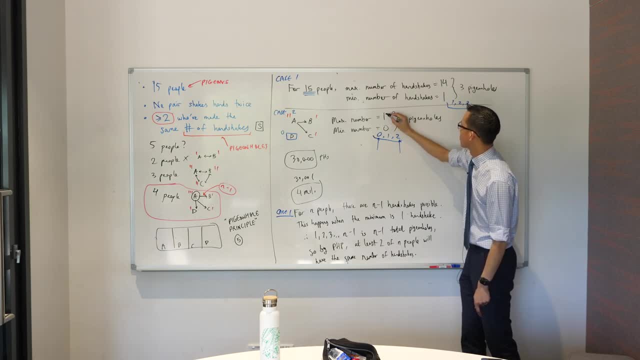 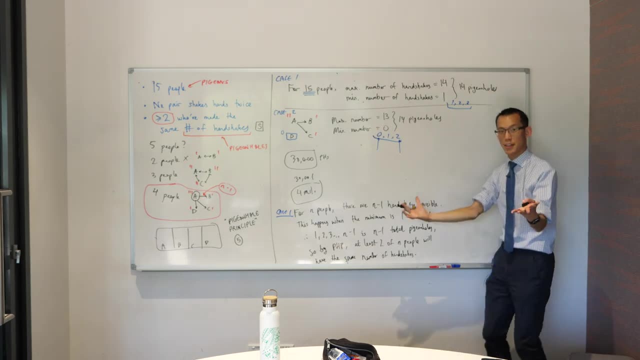 it would go all the way up to 15.. Okay, Um, 13 to 0, so it would be, in this case, 14 pigeonholes. in this case, still 14 pigeonholes. but I've got 15 people and that's it okay. 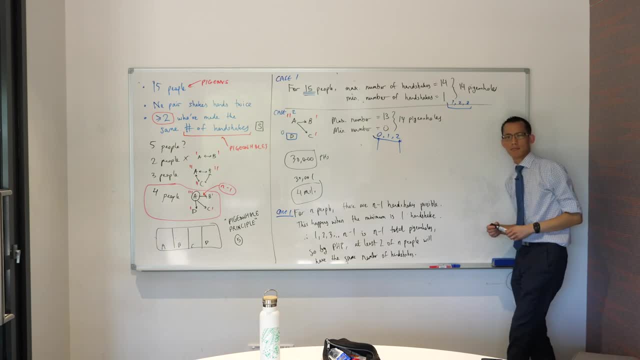 So this is in much the same way as sorry, have you guys done? you guys would have done series and sequences right. You've done that. have you already? you've already met some of it, Yeah. So in much the same way that when you have to establish a series right, you need say, for example, 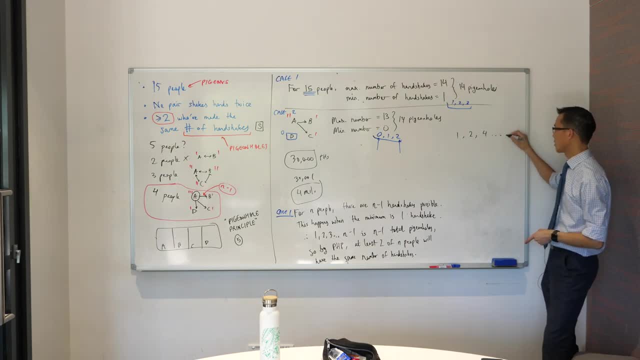 you need 3 terms, right, And then after that you can say 2 to the n Pattern's established off, I go right. But you can't go like 1, 2 to the n, right? You actually have to show the logic that's going on there. 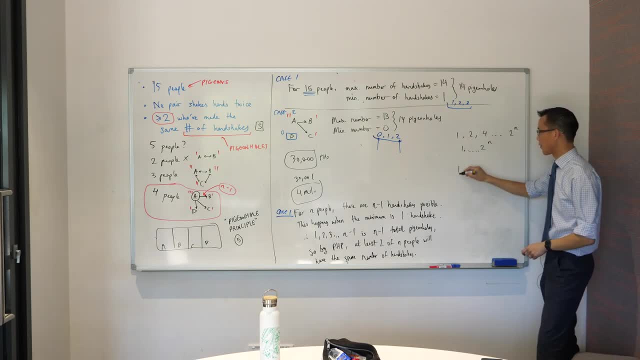 And the reason why 3 is the magic number is because if I gave you 2, this could be arithmetic or it could be geometric, right? You're like you really don't know, okay, And it's the same thing with this. 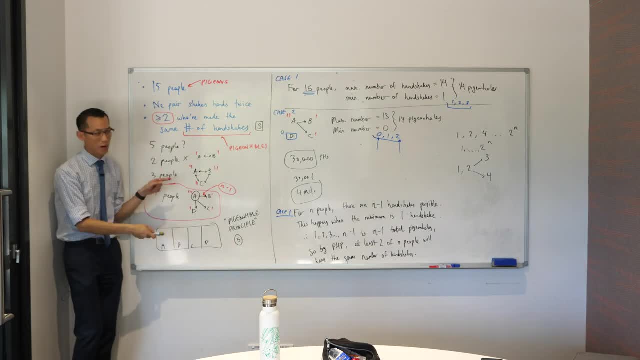 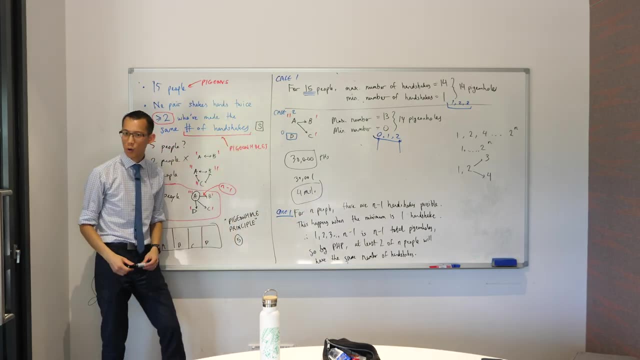 I haven't actually established a pattern yet until I get to this point, And then I can say: oh, the word for this, by the way, is called generalizing Right, And that's why I've got all these n's and n minus 1's here. okay.